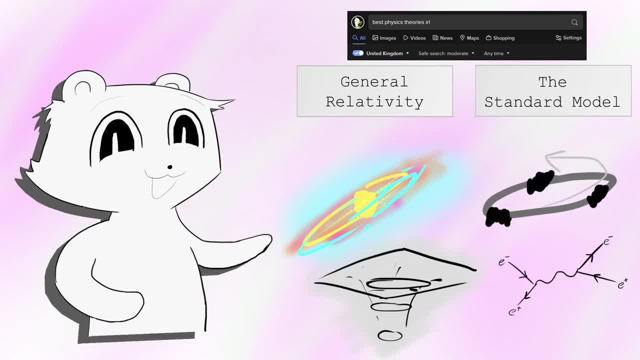 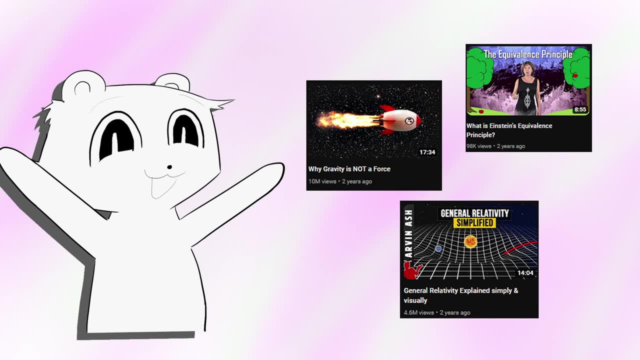 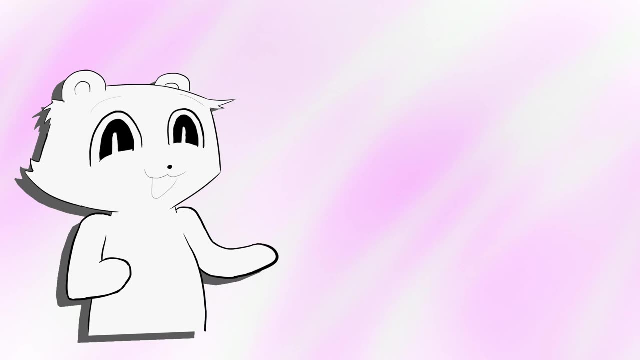 systems and galaxies, and one for tiny scales like atoms and particle colliders. While general relativity has enjoyed mainstream popularity, with everyone under the sun trying to convey the essence without its mathematics, the same can't be said about the standard model. It's quantum, so it doesn't make any sense. seems to be the mainstream sentiment. 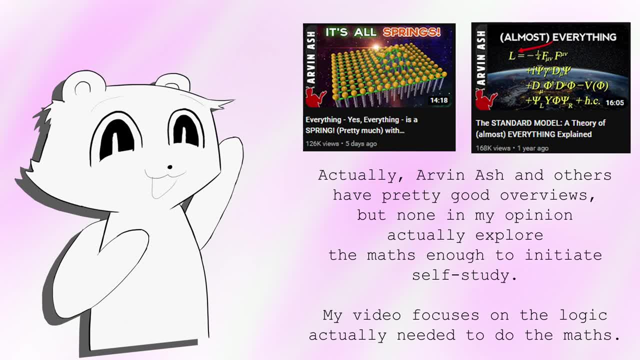 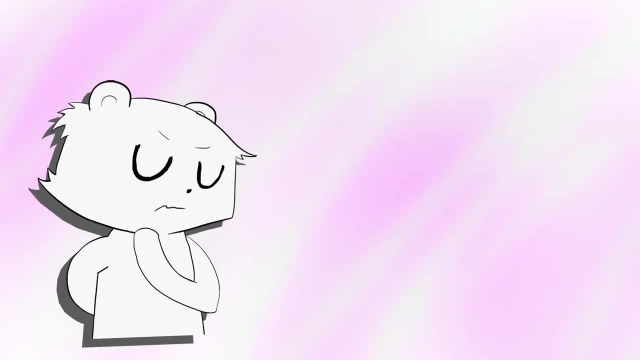 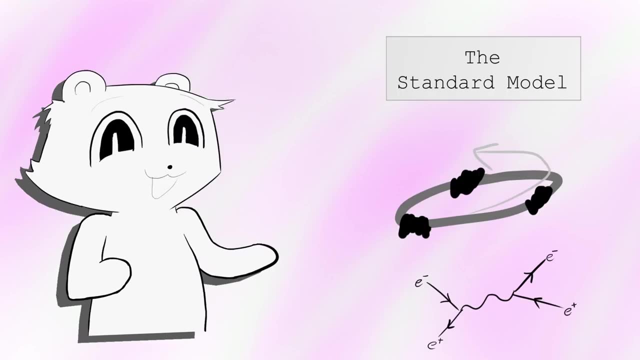 Not a single sexy animation exists to share its revolutionary concepts to anyone without a four-year course of mathematics. What are Feynman diagrams for? What is quantum field theory? What is the logic underpainting the most accurate and useful theory of quantum theory? What is the logic underpainting the most accurate and 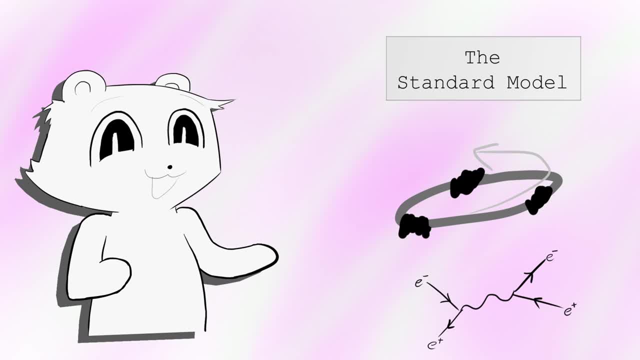 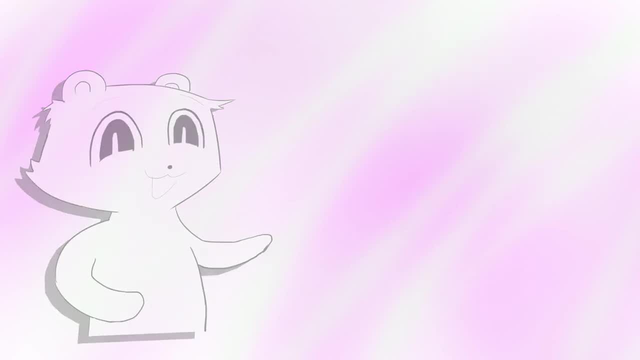 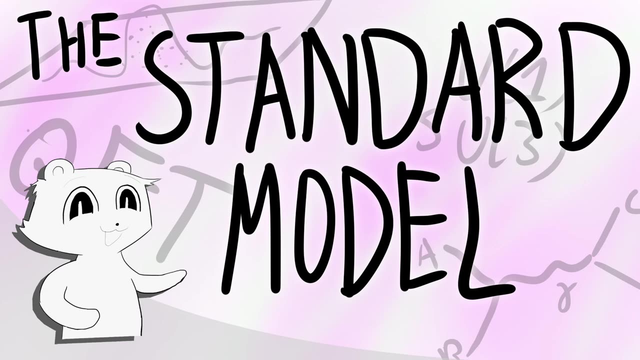 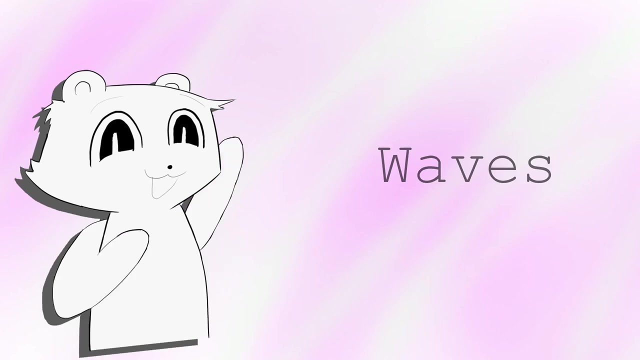 predictive theory in all of physics have to say about the universe in which we live in. That's what I want to talk about today. This journey begins with waves. Let's have a brief review. At A-levels, you've probably learned of waves as wavefronts. Each wave is 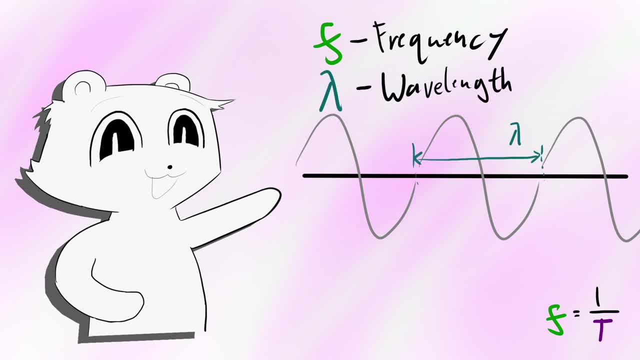 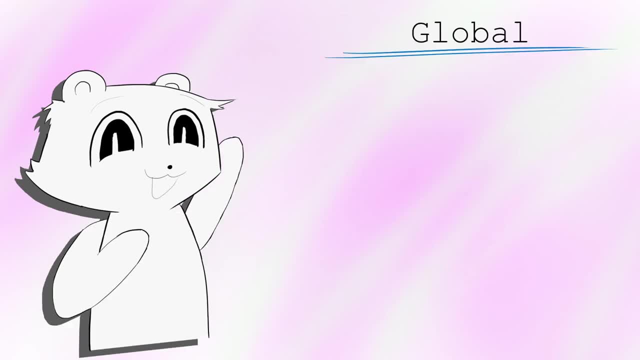 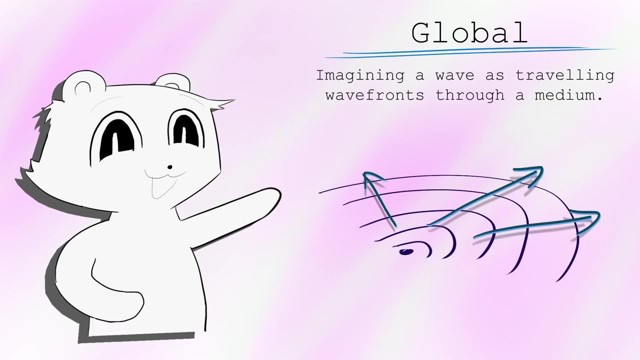 described by its frequency, its wavelength and its phase. They can constructively interfere and destructively interfere. This way of understanding waves is called the global perspective of waves. It's global because you're looking at the entire wave in one go, But there's an equal and in some cases, more powerful way of looking at waves: The local view. 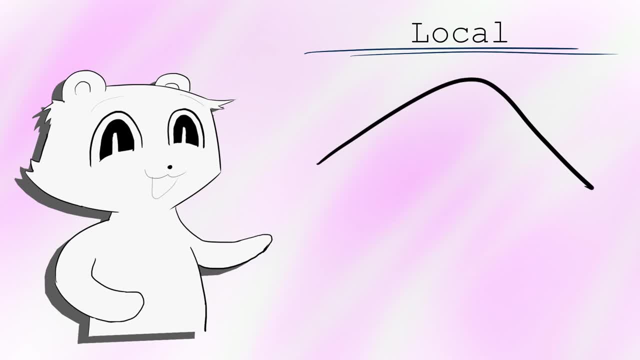 If we imagine a string and that string is being stretched by some amount so it has some curve at that point, then the string around it is going to restore this string so it becomes straight. This is the natural tension that exists in all strings and you can see it whenever you play. 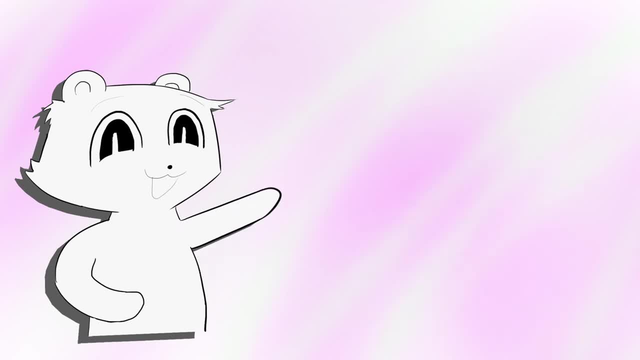 guitar. If we look at the mathematics describing this, we get this: The second derivative of space, which is the curvature of the string, is negatively proportional to the second derivative of time, which is the acceleration of that string. There are a surprising number of ways you can interpret the wave equation. 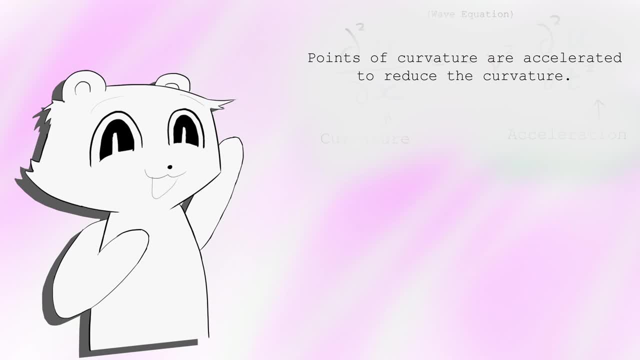 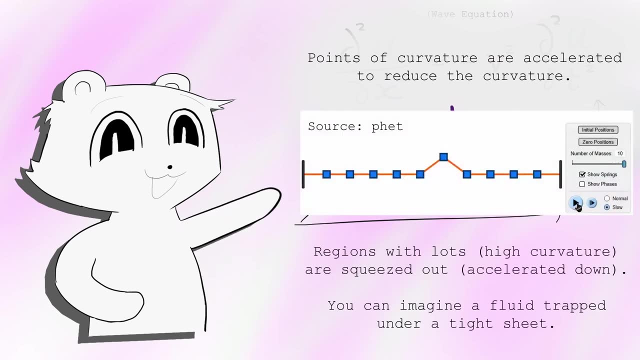 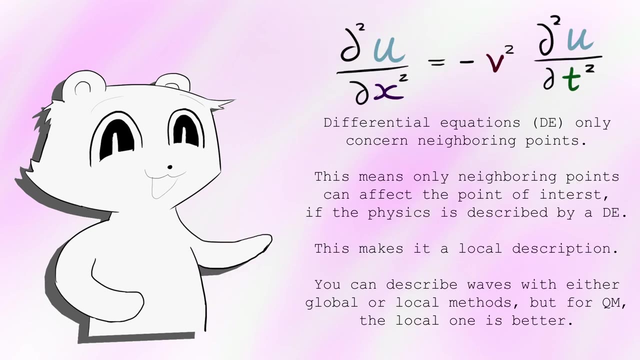 but the one we'll be using today is the idea of squeezing. Curvature in this case can also be interpreted as this point has a lot more than its neighbors. If you're curved downwards, then, by definition, all your points around you are smaller than you. This local or differential view of waves is important when it comes to. 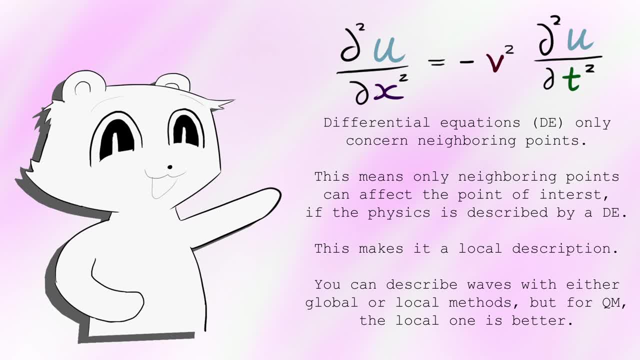 understanding quantum mechanics, because quantum mechanics describes particles as waves. So let's look at this again: We're trying to explain a wave in a different way and we're trying to understand it in a different way. so let's look at this again: We're trying to understand a wave in a different way. 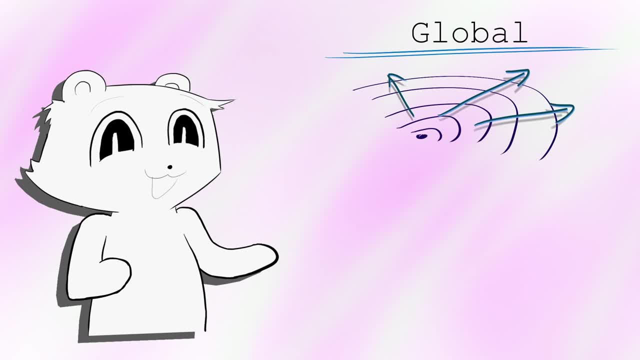 and we're trying to understand it in a different way. so let's look at this again. We're trying to understand a wave in a different way. We rarely care about the massive wavefronts. we care about how particles move at the very. 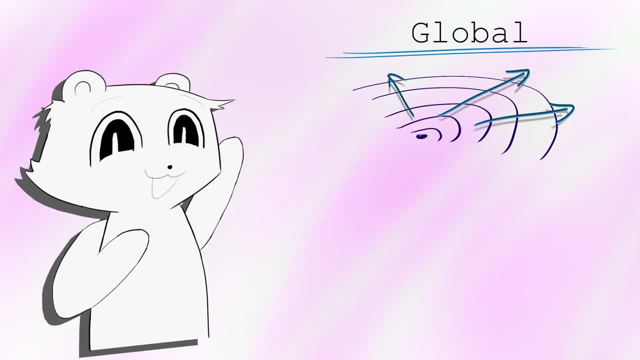 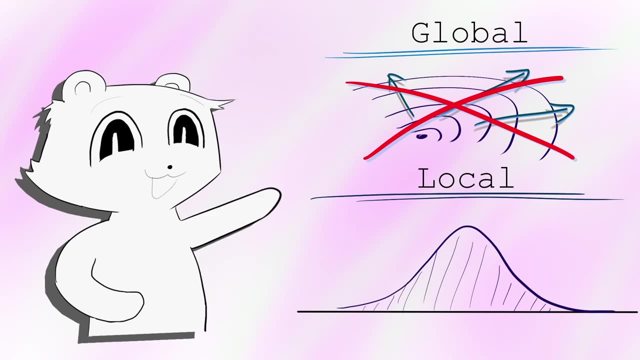 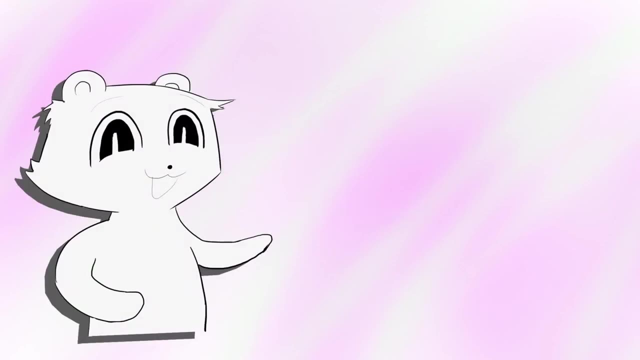 tiny scales, And in that sense trying to imagine particles as massive waves is incorrect. It's more intuitive to think of quantum particles as being particles that want to squeeze themselves in every direction. So with that out of the way, let's look at the Standard Model. 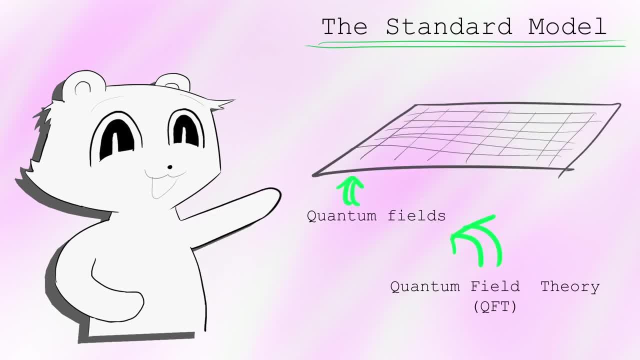 The Standard Model uses quantum fields. described by quantum field theory, A field is just like an empty pond: Particles are ripples upon that pond Kurzgesagt made a lovely video animating it in more detail, which you can watch here. 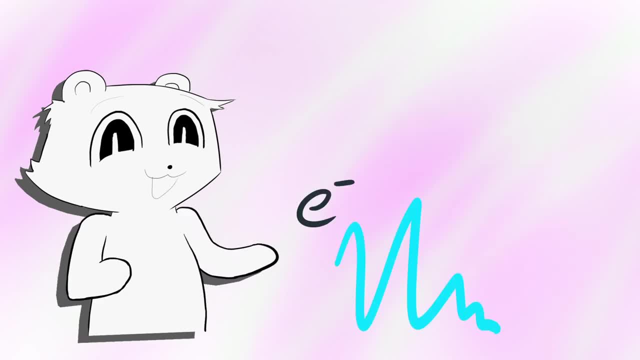 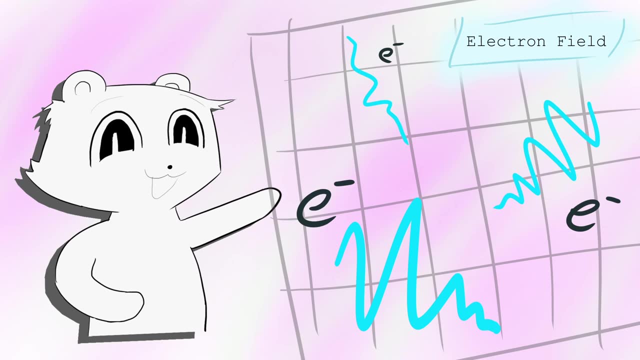 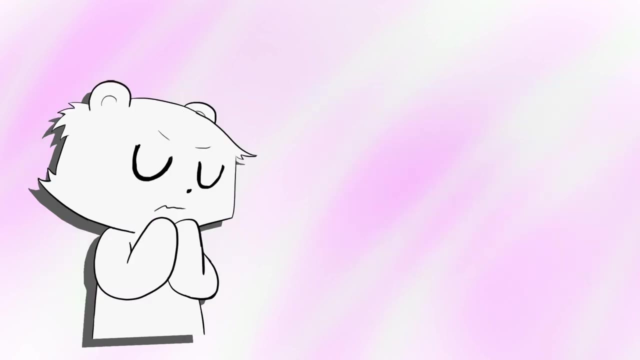 This is the reason: all electrons are identical. You're not observing a million different electrons. you're observing ripples on the singular electron field. Imagining fields instead of particles makes particles, wave nature, intuitive. Think about it like this: A particle doesn't have a memory. it doesn't know which direction it came from or which. 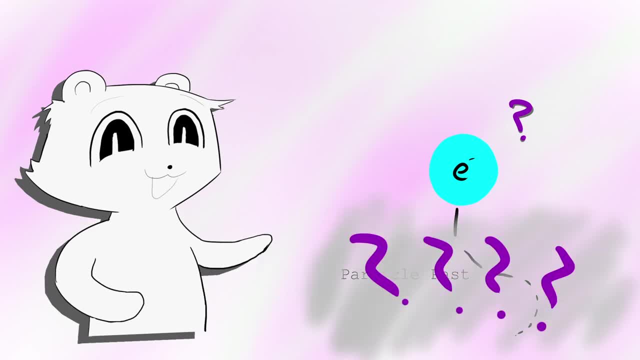 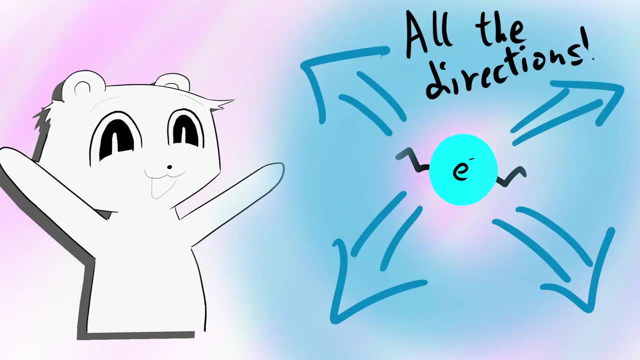 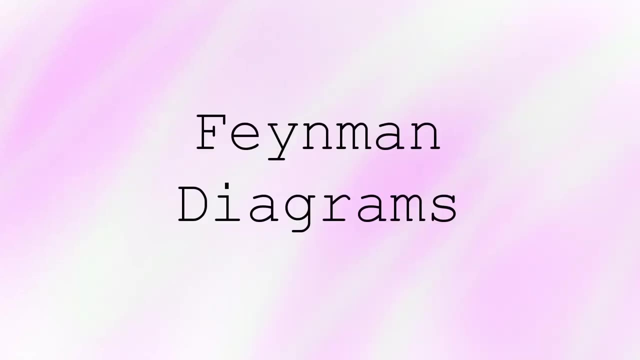 direction it should be going, Because a particle can't see its past, it can't continue its path and therefore it travels every possible path that it physically can. We have just predicted the wave nature of particles. Okay, okay, okay. 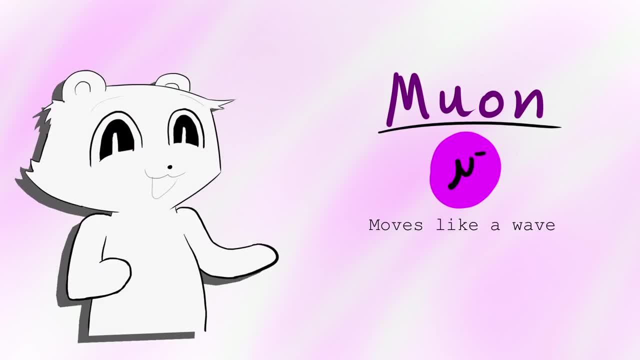 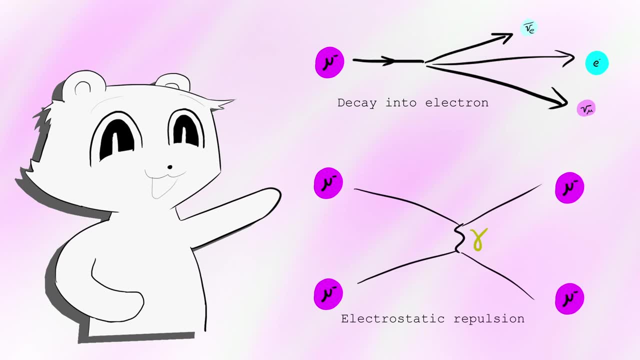 Particles are waves- cool, that makes sense. But particles do a lot more than just move like waves. Particles don't do nothing. They decay. they interact with other particles through forces and all of this other humbo-jumbo. 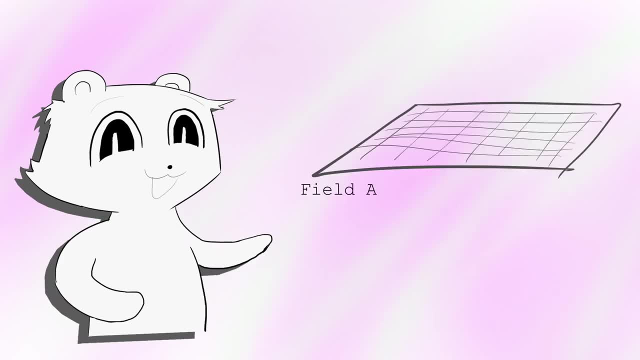 What does this come in? Well, it comes to the idea that particles don't just flow through space and time, They also flow into other fields. Let's imagine two one-dimensional fields. One field can flow into the other field. We start off with a pure pulse in one field. 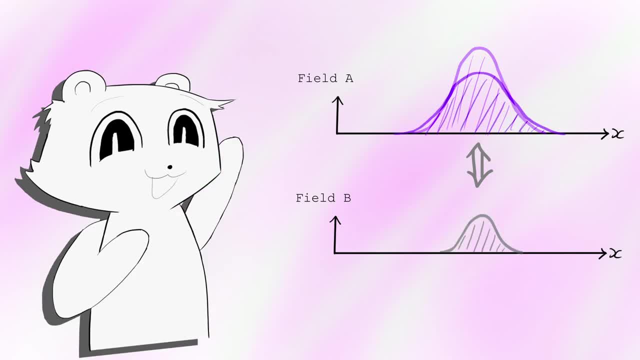 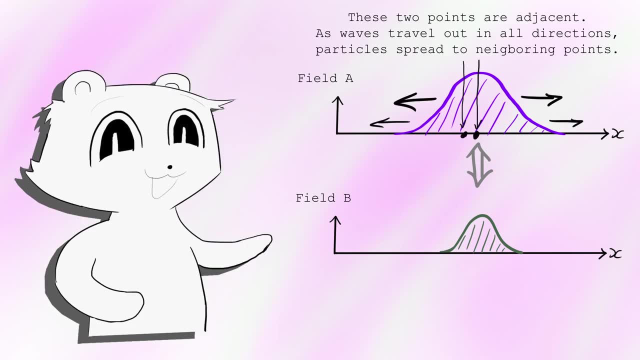 And over time, as it flows forward through time, it also flows into the second field. Now think of what a particle is actually doing. A particle is just trying to travel in every direction it can. If a particle is able to move into another particle, it means that those fields are in. 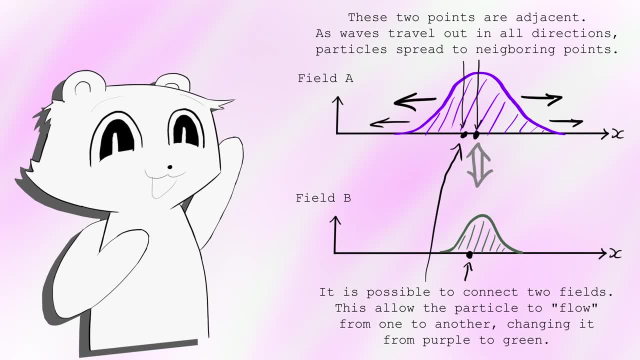 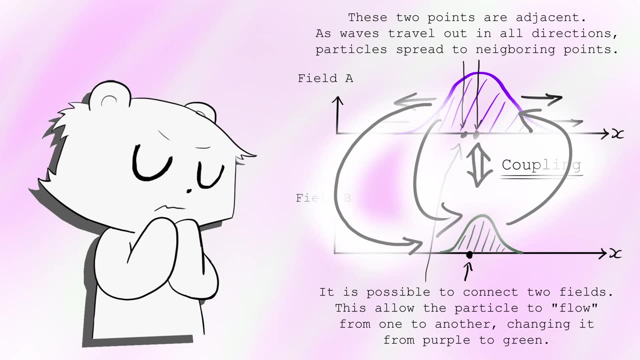 some way linked. The same way the two adjacent parts of space Are linked. We call this coupling, And if field A is coupled to field B, it also implies that field B is coupled to field A Now because it's waves. wave A could turn into wave B, which could turn back into wave. 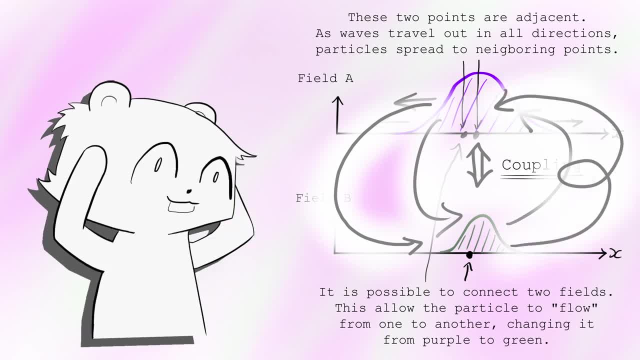 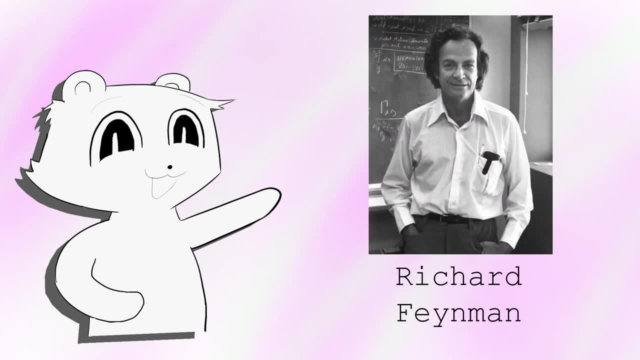 A or stay as wave B, and you know it's a right mess. To keep track of what's going on, a very smart person named Richard Feynman came up with diagrams to keep track of where the wave is going. 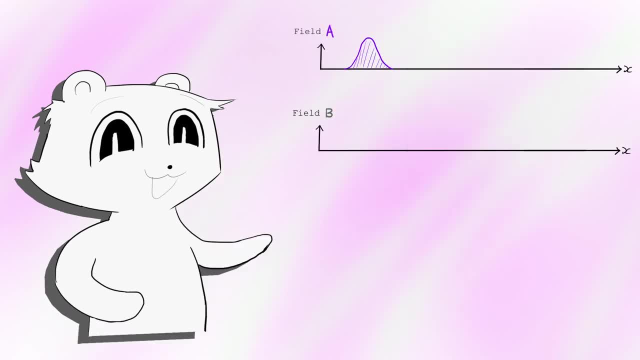 To see how he did this, let us look at the example of our two fields. First of all, what would happen if the fields weren't coupled? Well then, the particle in field A would just go on forever. We write this in our notation as a straight line. 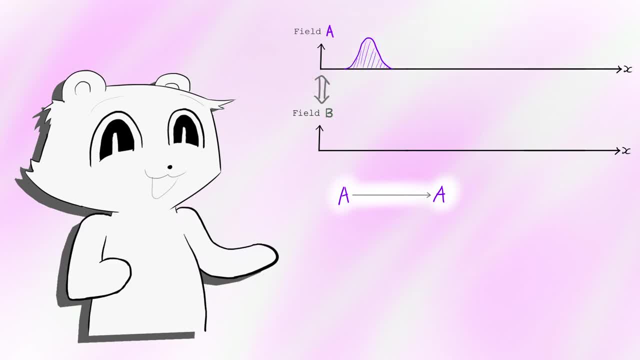 The particle A moves as particle A. Now what would happen if the particle turned entirely into particle B? Well, this depends on the coupling strength between the two fields, usually written as G In the diagram. We show off that particle A has turned into particle B by adding a vertex. 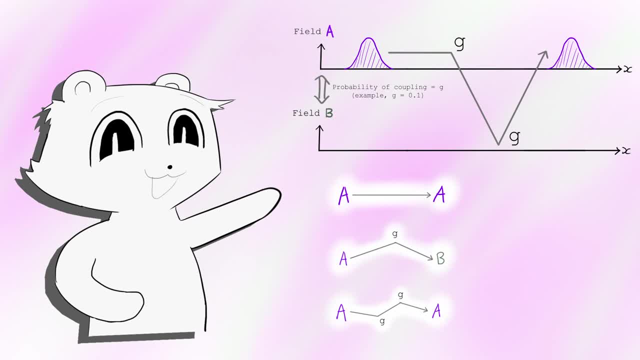 If the wave decided to turn back into particle A, then we have to add a second vertex. Each time we add a vertex, the chances of it happening decreases, as G is less than 1, and each vertex adds a multiple of G to its probability. 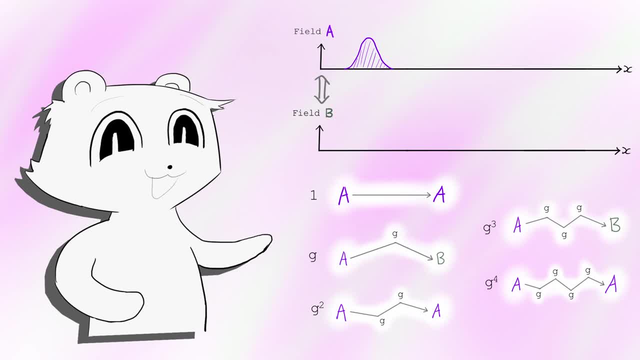 Now, the reason why I'm showing all of these diagrams at the same time is because remember what we are actually trying to describe. We're trying to describe a wave. The wave is going to go every direction. It's taking all of these paths at once. 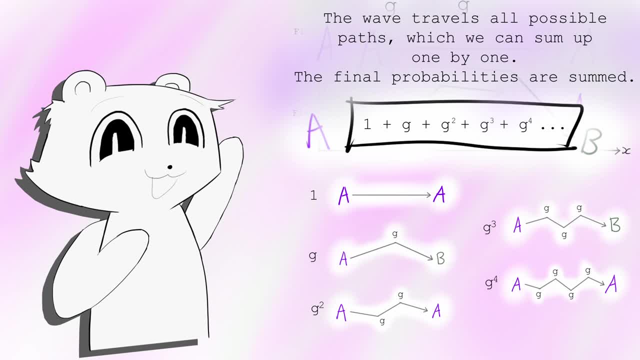 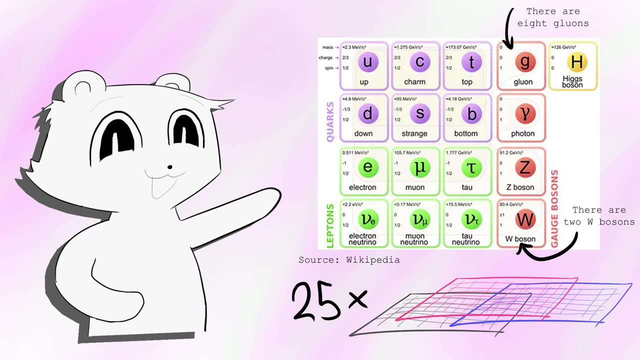 This is why the final step of any Feynman diagram calculation is to sum all Feynman diagrams together, Because that is the true path of the wave. There are 25 fields for the 25 different particles in the standard model. We get the rules for these fields. 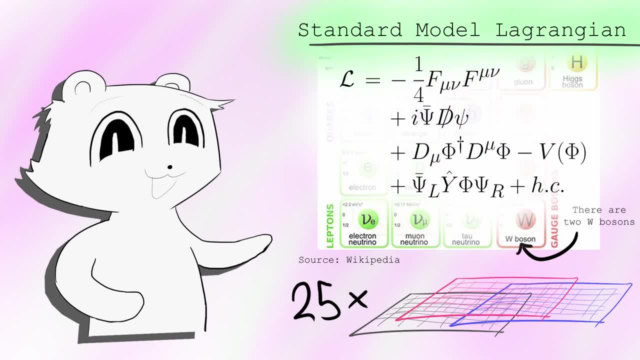 For example, we have to find out how many of these particles are in the standard model Lagrangian. Now a lot of symbols are going to appear on the screen, but surprisingly, you don't need a lot of maths to understand it. 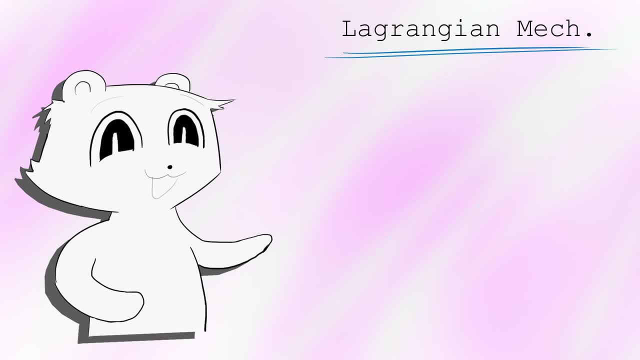 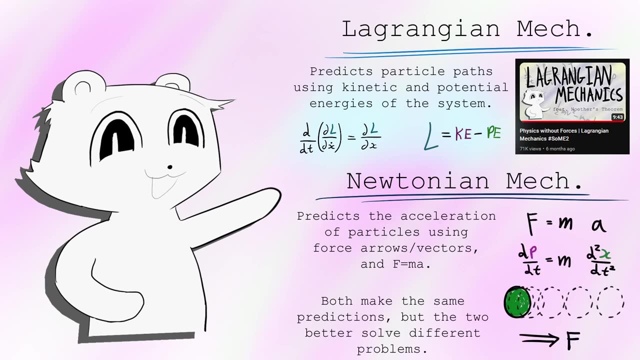 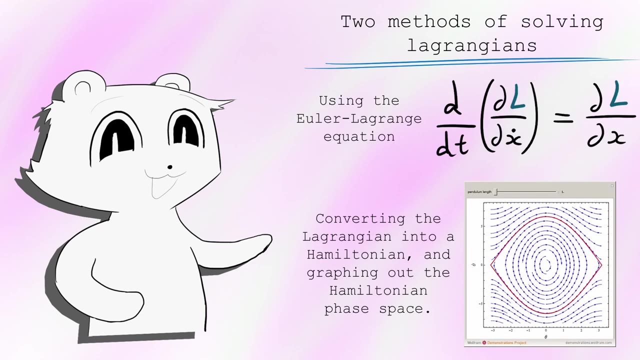 Just follow along, okay. Now, if you've done Lagrangian mechanics at university or even just watched my video on it, you'll know about it as an alternative way of doing Newton's mechanics. We do this by using Euler-Lagrange equations or by plotting the Hamiltonian phase space. 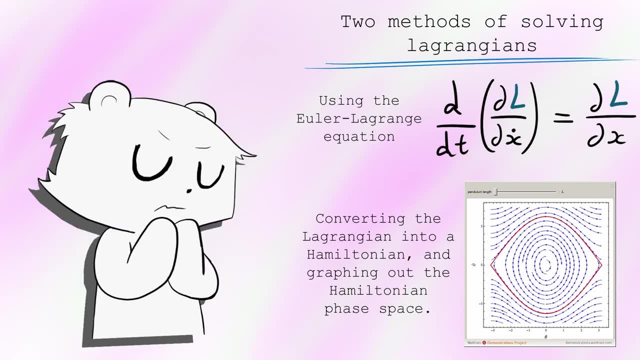 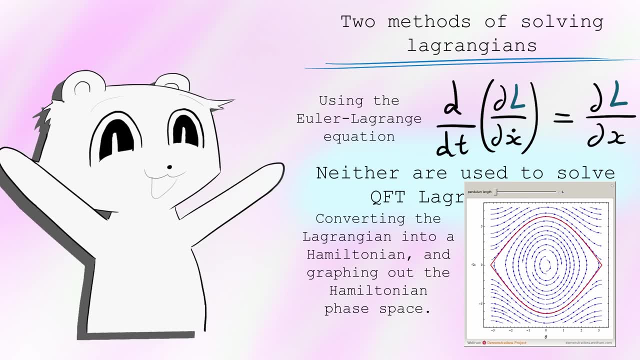 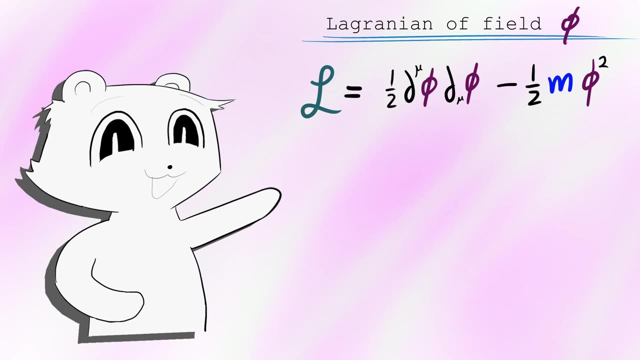 and then working through the calculations. Interestingly though, none of those mathematics are needed to work with quantum field theory, And I'm going to show you how. Let's look at a simple example. This is the Lagrangian of a massive scalar field. 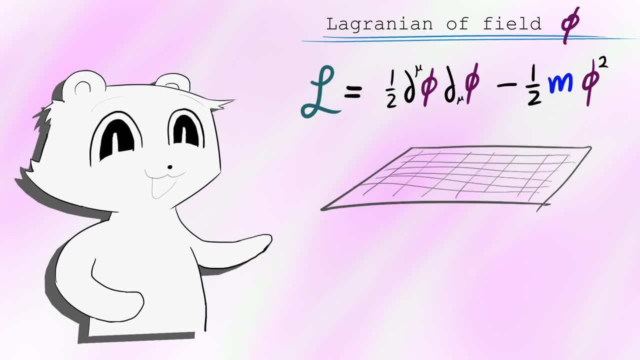 Remember it's fields that we're describing here, not particles. This single equation can describe zero or an infinite amount of this particle. The Lagrangian is made of two terms. The first one is the kinetic energy, The second is the mass term. 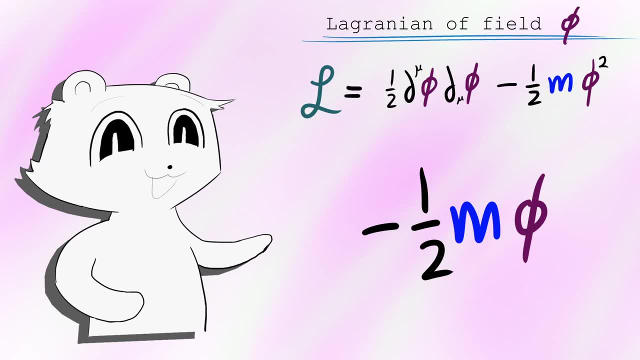 Out of the two, the mass term is the easier of the two to describe. M here tells us the mass of the particle. If the mass of the particle is zero, then this term goes to zero. Therefore, if this term just wasn't there, then this particle is massless. 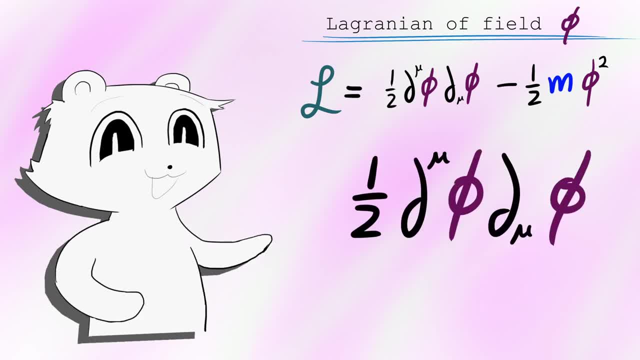 Mystery solved. The kinetic energy term, on the other hand, is a bit more interesting, because it is allowing this particle to move. Now you might be thinking, oh, without this term, the particle is just stuck there, I can't move it. 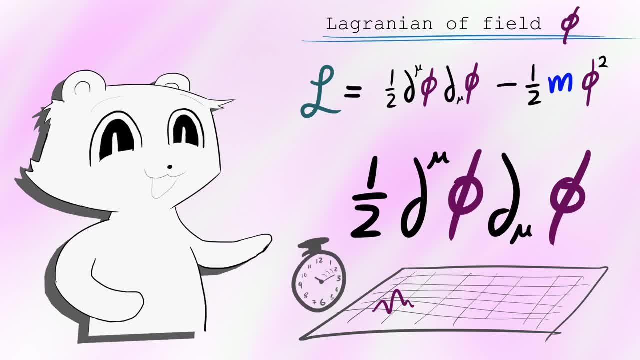 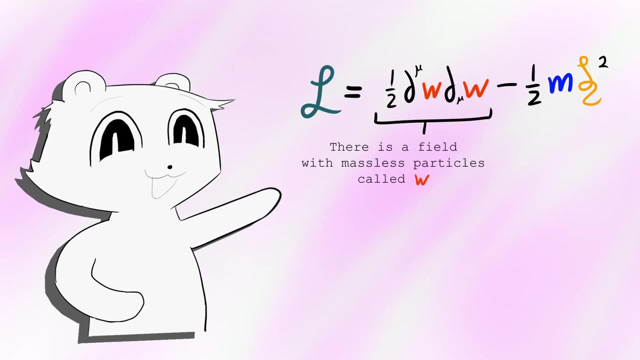 But remember, moving through time is moving as well. We're working with spacetime. after all, time is another dimension. Therefore, the kinetic energy term really should be called the existence term. If we find a kinetic energy term, we know that that symbol right there, that's a field. 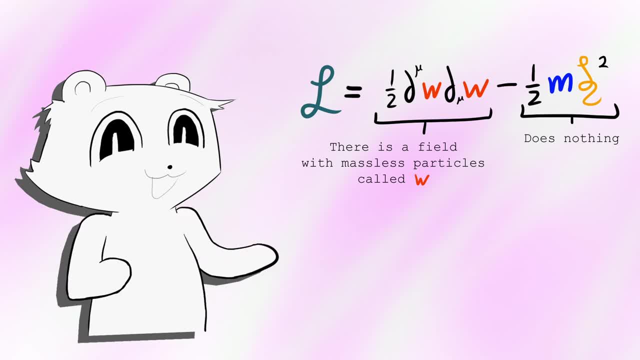 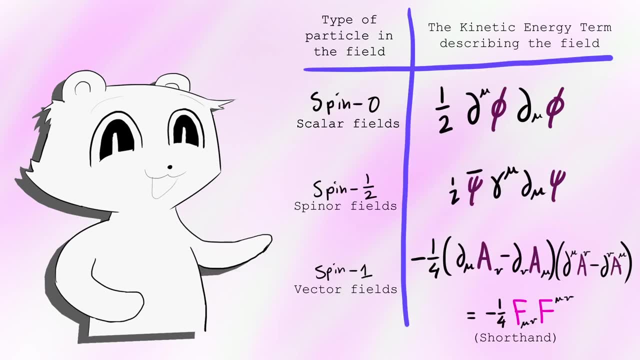 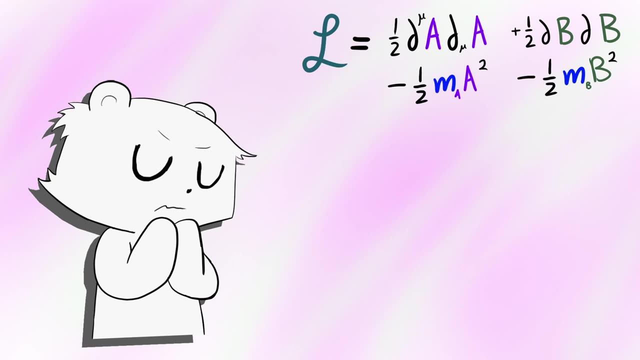 Even if I had a mass term for another field, if I can't find a kinetic energy term for that field, then this mass term does nothing. Conveniently, there are only three kinetic energy terms that you find in the standard model. But a Lagrangian with just kinetic and mass terms will do nothing. 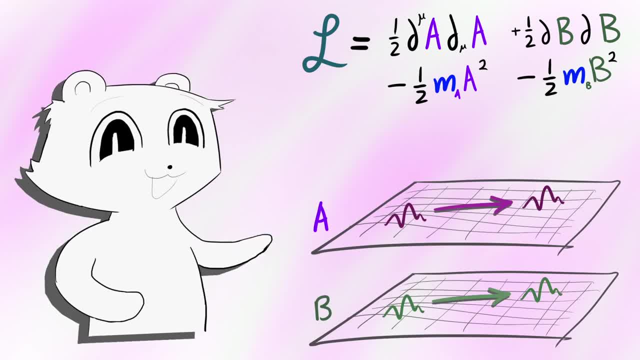 These fields don't do anything aside from move. Let's use the example from before: This is my field A and this is my field B. Now, this is Lagrangian mechanics, so in order to add new physics, I just have to add a term. 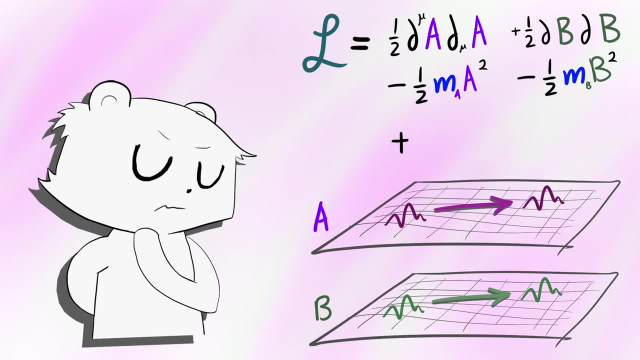 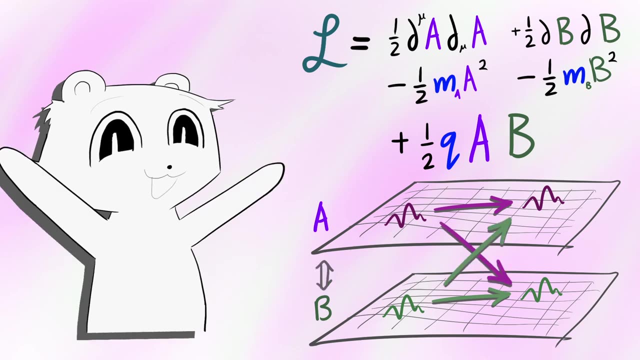 Now, what kind of term would couple these fields together? Well, this term has to include A and B, And look at the mass term. there's probably a variable in front. So with that reasonable guess, we have QAB. This is our interaction term. 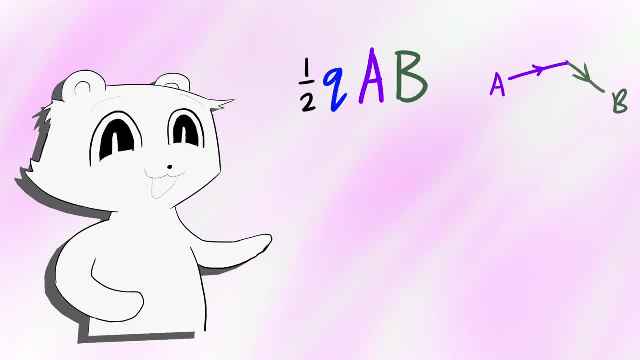 Specifically, it creates the vertex 1A and 1B. It's possible to have more questions about this, But let's get to the point. Let's get to the point. Let's look at some more complex vertexes, For instance A squared times B. This produces this vertex in a Feynman diagram. 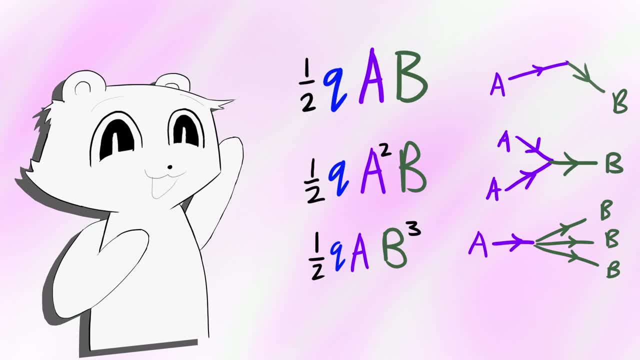 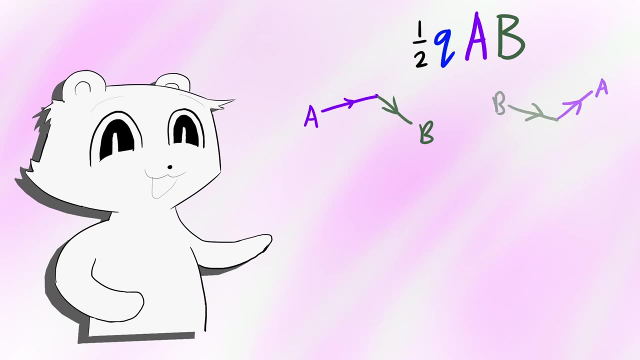 In general, any term that isn't the kinetic energy or mass term is an interaction term and these interaction terms allow fields to flow into other fields. By reading off the powers of the interaction terms, we get our vertex Also, because this is coupling, it doesn't matter which way around the particles are. 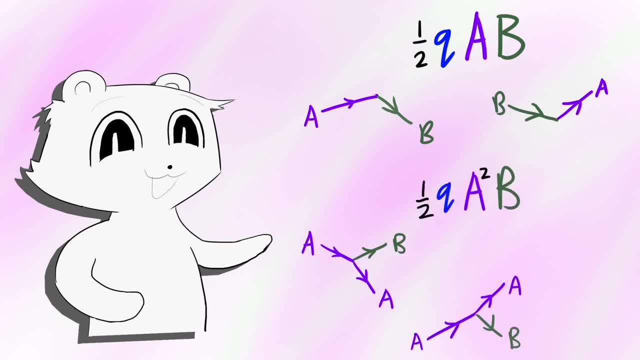 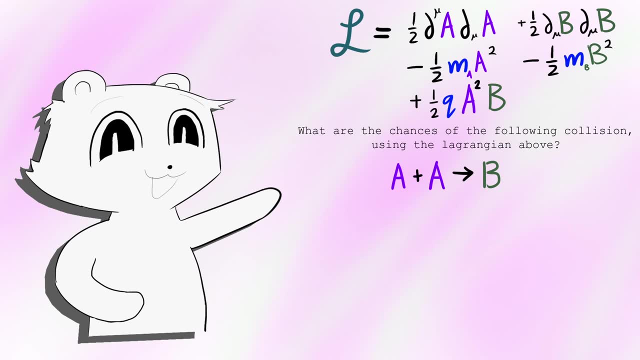 going A turning into AB or B turning into AA. You can just rotate the vertex By reading off of the Lagrangian and constructing Feynman diagrams. we can actually skip calculating with the Lagrangian entirely. This is what Feynman was so famous for. 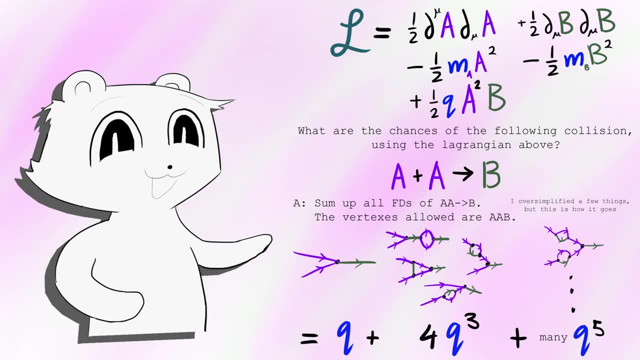 The use of Feynman diagrams allowed people without a ridiculous understanding of maths to do quantum field theory, And it was this innovation that pushed physics to its fattest potential. And it was this innovation that pushed physics to its fattest potential. It was this innovation that pushed physics to its fattest potential. 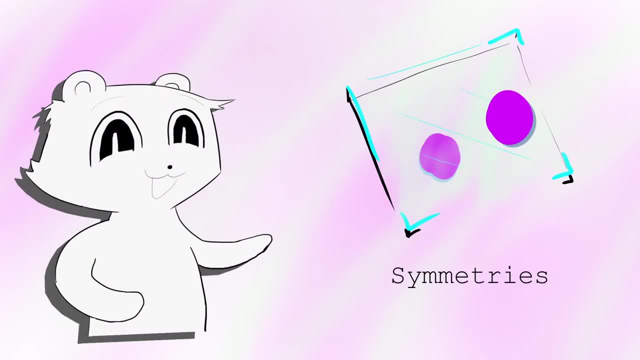 fullest potential. The final part of this video is going to be on symmetries. First of all, particle physicists call symmetries gauges. for whatever reason, If you see stuff like gauge forces or gauge particles, it's better to think of these as symmetry particles and symmetry bosons. 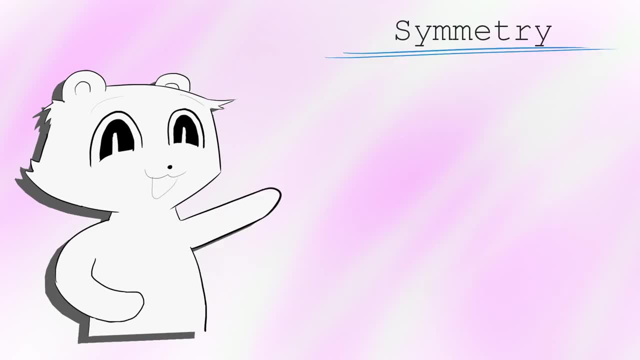 What does that mean? Well, watch the rest of the video. There are lots of ways that something can be symmetric. It can be symmetric along reflections or symmetric along rotations. As long as something looks the same after a transformation to it, it is symmetric. 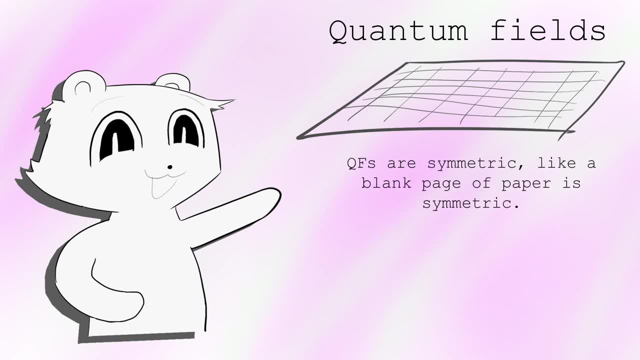 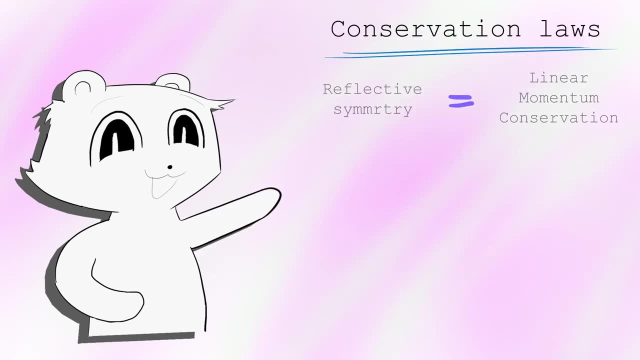 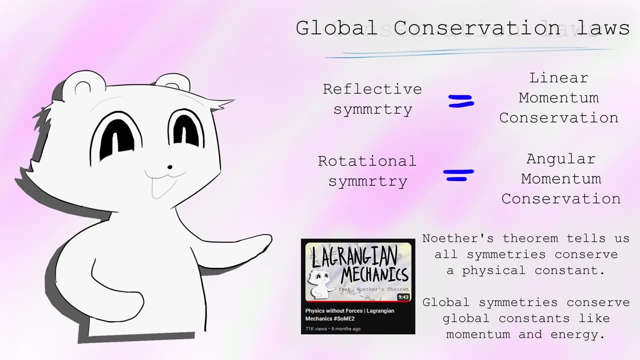 Obviously, all fields are rotationally and reflexively symmetric, Not particles fields, While this universal symmetry gives rise to linear and angular momentum conservation. more details can be seen in my Allegro and Geomechanics video. these are examples of global symmetries. 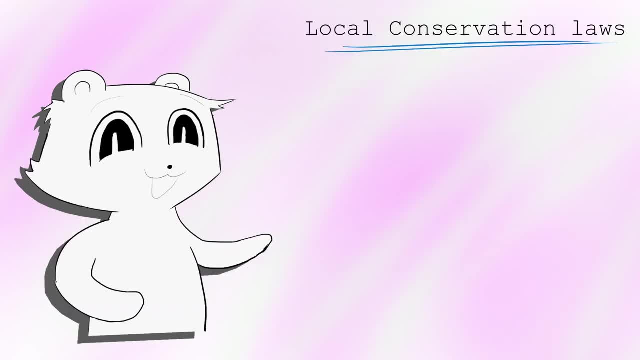 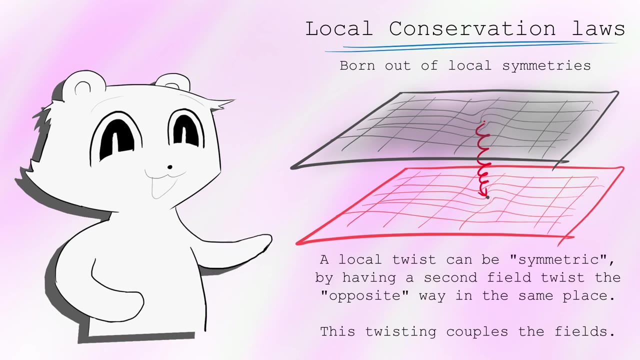 There are symmetries of the entire field, It is also possible to have local symmetries. We can imagine a local symmetry as a certain twist we can do on the field. This twisting gives particles new pods to go, Of course, if a particle is going to another field. 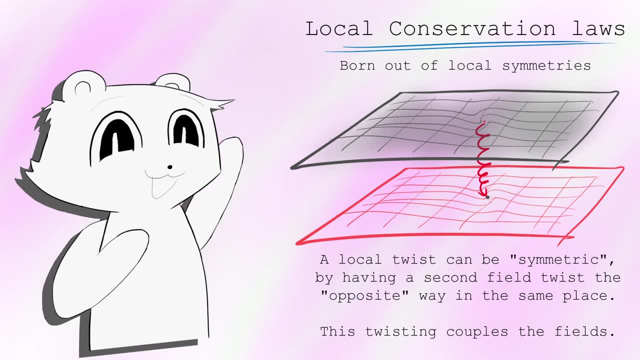 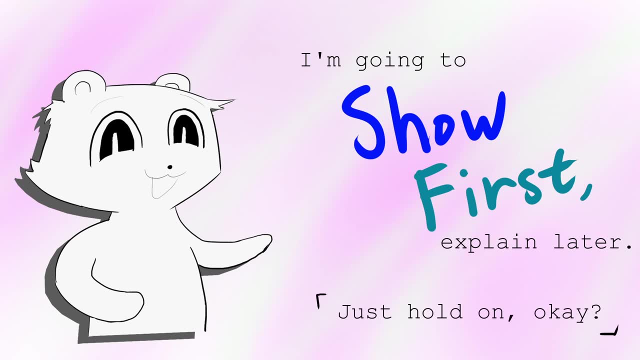 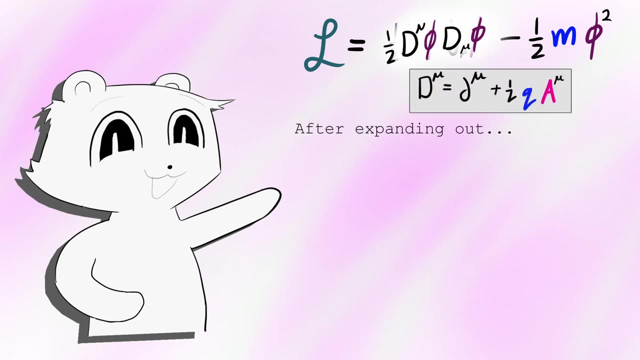 it is coupling to this field. Symmetries are a way of introducing couplings to existing fields. Let's see how the mathematics turns out. We start off with the free-field Lagrangian. We substitute all partial derivatives with covariant derivatives, We expand it out and this is what we get. This is the familiar kinetic energy. 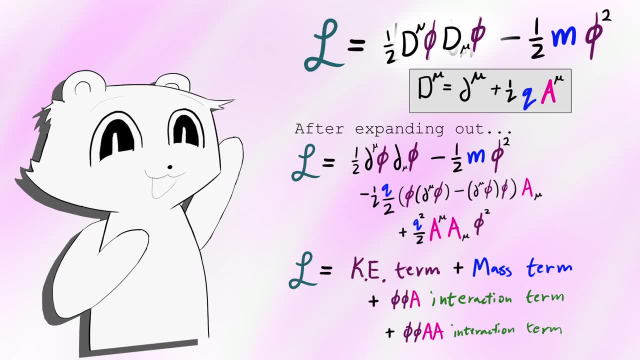 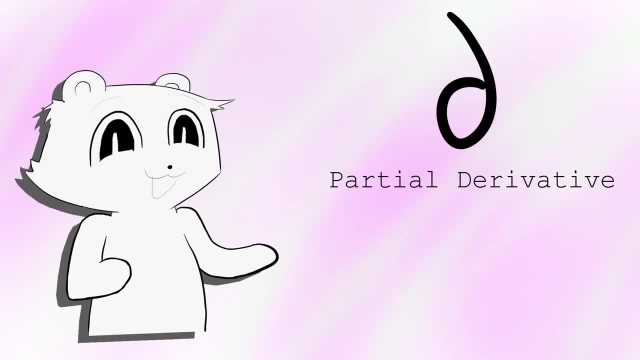 and mass term, and these unfamiliar terms are our interaction terms. Now we need to spend a few minutes understanding why. What is the theoretical power of a derivative? In maths we see derivatives as tools. We get other functions out of them, But in physics, derivatives have a very specific purpose. 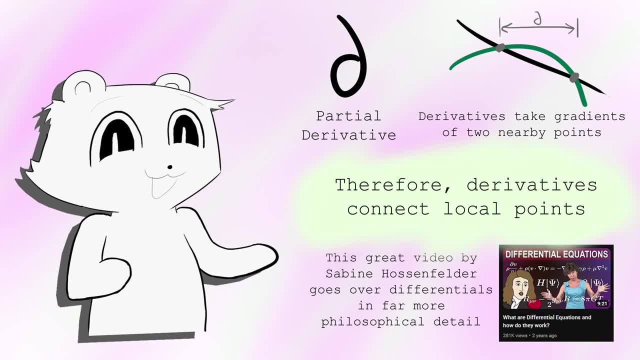 They connect bits of space together. Without a derivative of space, we can't say how something changes through space. Without a derivative in time, we can't say how something changes through time. Therefore, when we come up with the idea of adding in a new way to go for this, 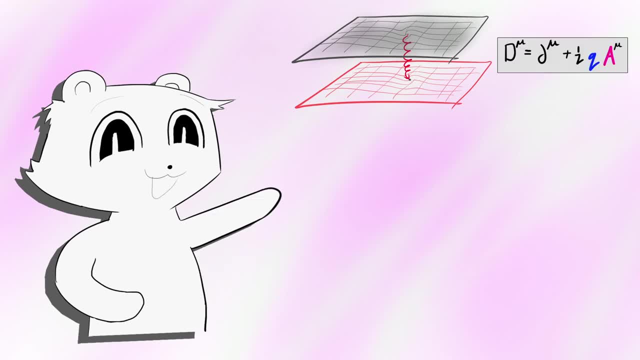 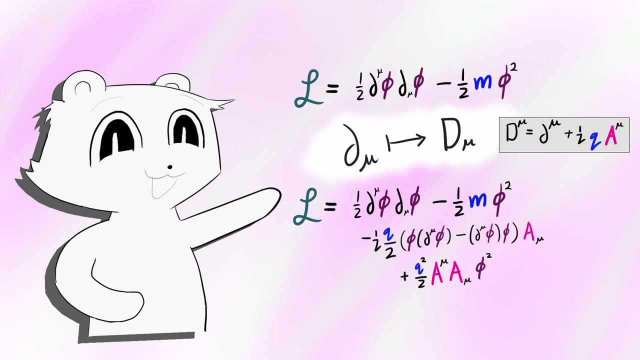 particle. we do this through the derivative. Derivatives are usually symmetric through space and time, But covariant derivatives are specific derivatives that are symmetric in additional ways. This method of blindly substituting our partial derivatives with covariant derivatives is called minimal substitution. The keen-eyed among you might realize that this field on its own, 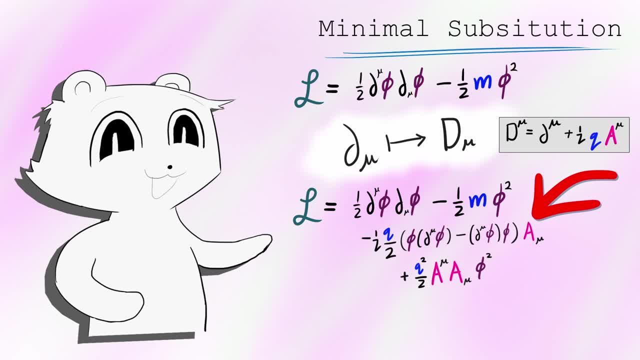 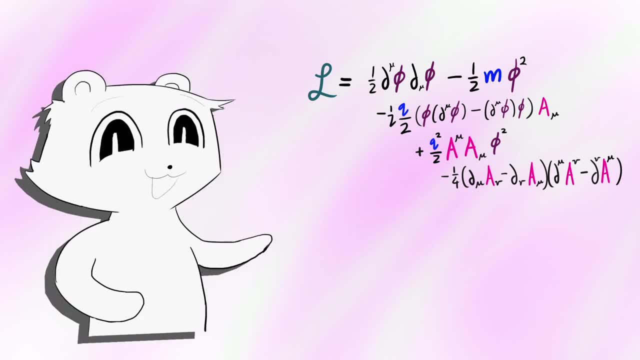 can't do anything, Since this new field is spin 1, we add the spin 1 kinetic energy term. Hold up: This is the exact field equation for electric Support. Hold up, Hold up, This is the exact field equation for electric Support. 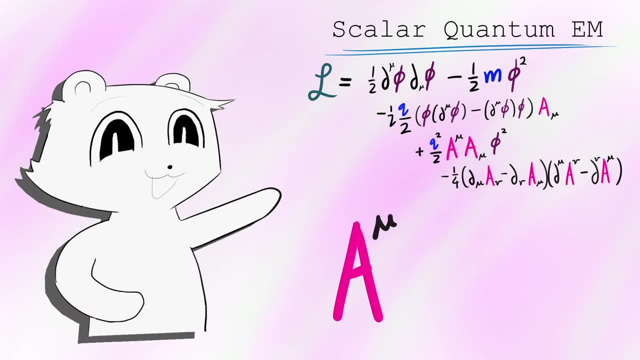 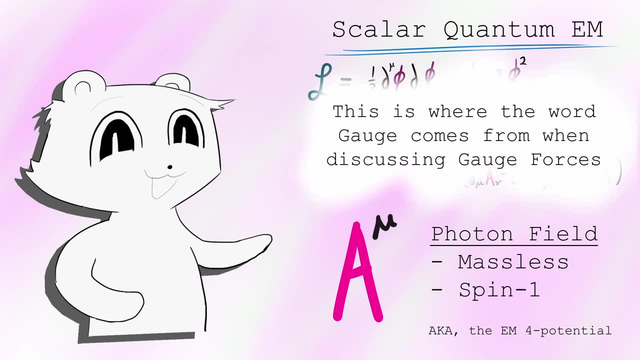 Hold up. This field A is literally the field for photons. These fields, which were born out of symmetries, are what we in everyday life call forces. Therefore, we call these fields symmetry force fields or gauge force fields. This is how particles are actually coupled. 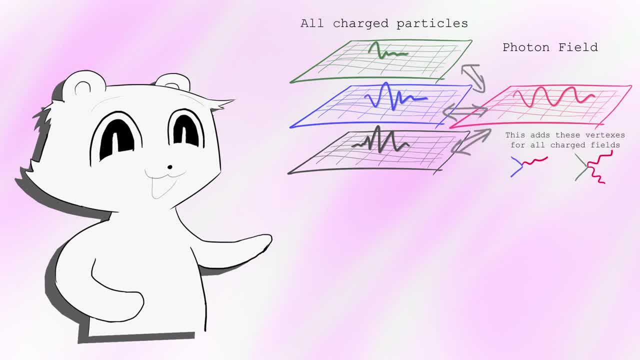 It's extremely hard to just force one field to couple with another, but it's really easy to have all of your fields coupled to force fields and having all your particles interact through this middleman field. By identifying all the fields and coupling to the right forces, we are able to predict. 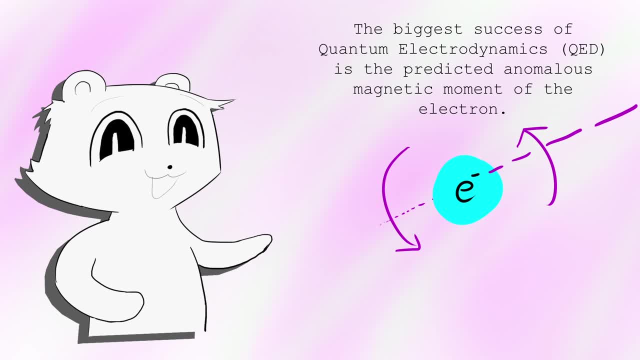 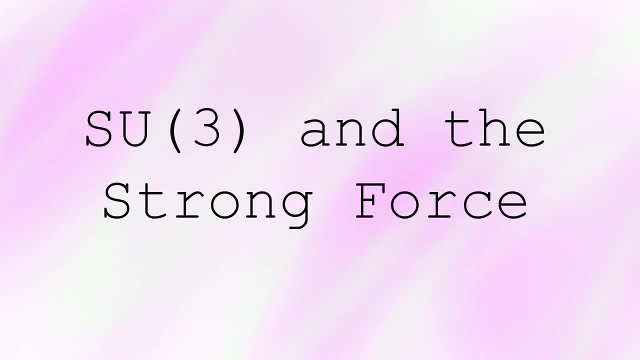 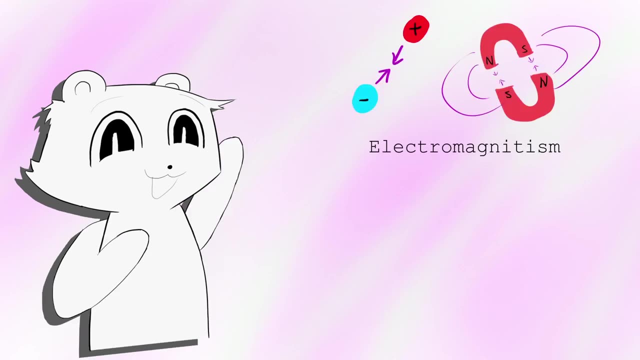 the electron's anomalous spin to 12 significant figures, The most accurate theoretical prediction in all of modern physics. In the standard model, there are two forces that are directly described by symmetry: Electromagnetism and the strong force, modeled by U1 and SU3 respectively. 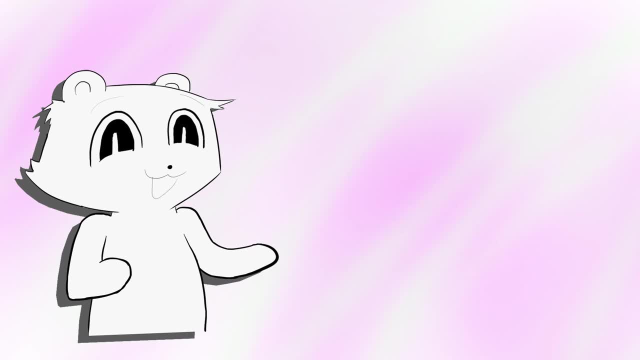 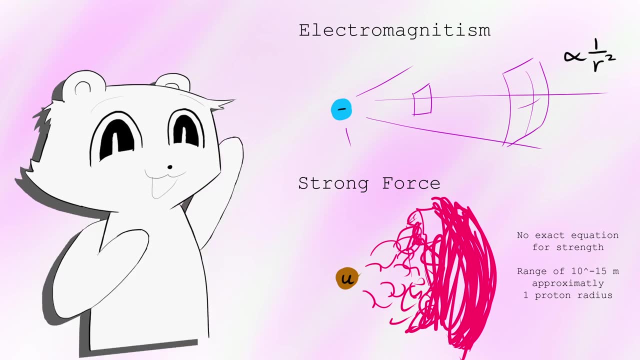 On the surface this seems fine, but for anyone who learns a little bit of particle physics, you'll know that electromagnetism and the strong force are completely different. Electromagnetism goes to infinity, with its strength dropping off by the inverse square law. 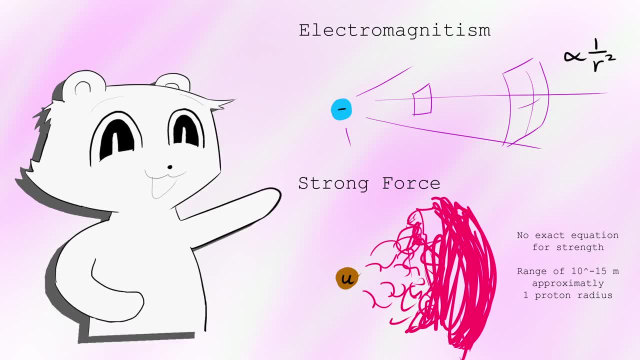 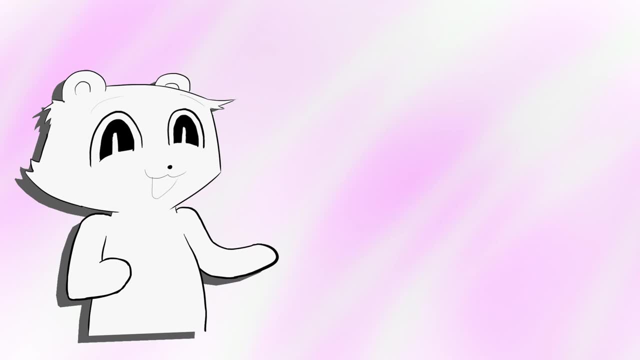 The strong force, meanwhile, gets stronger with distance and has a finite range. How can these two forces be described? in the exact same symmetry dynamics, It turns out it's possible to at a glance know that any force that comes out of a SU3. 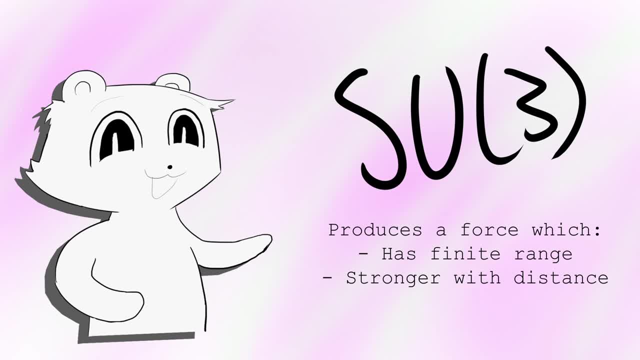 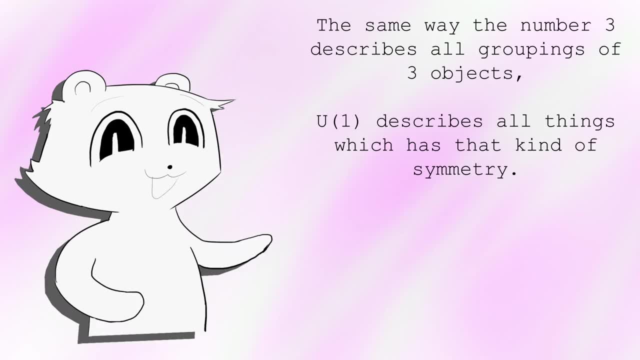 symmetry will have similar properties to the strong force, And to understand this we have to look at symmetries in a little more detail. When mathematicians say U1 or SU3, they aren't describing a singular thing that is symmetric, but instead a way that something even can be symmetric. 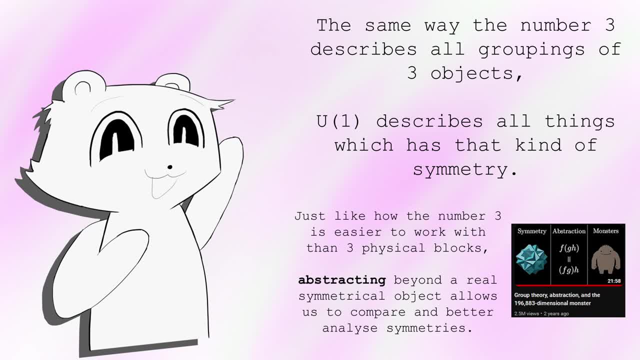 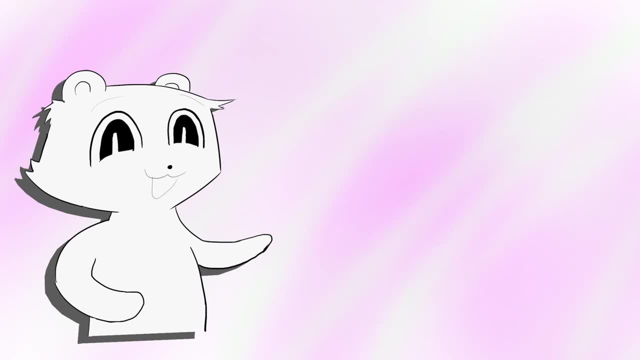 3b1b3.. John Brown made a beautiful video going over groups, which you can watch here, but for today I'll be focusing on a specific property that groups can have. Let's look at a very similar group to SU3, SO3. 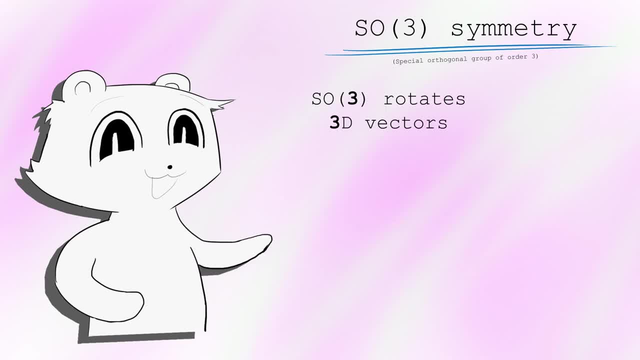 SO3 describes 3D rotations. If I have a vector in 3D space, I can rotate this vector using SO3 rotations. There's a special property that SO3 transformations have, and that is they are non-abelian. 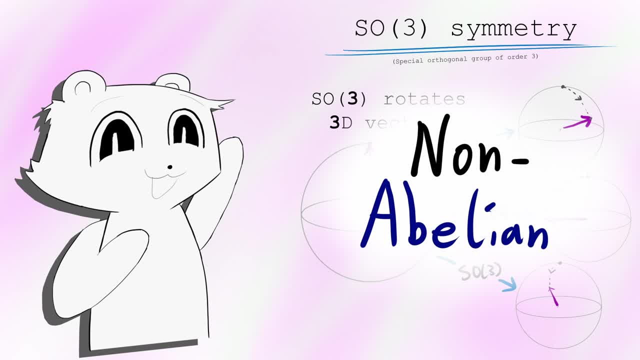 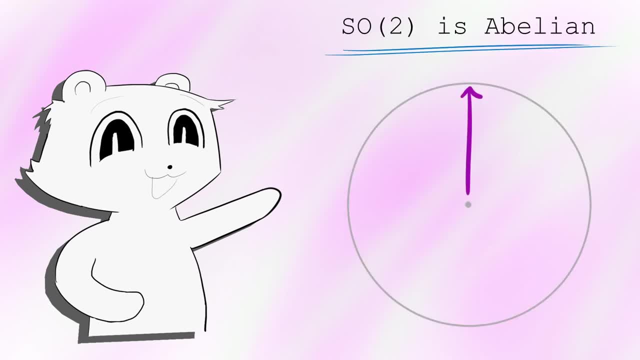 Abelian means you can do these symmetry rotations in any order. An example of an abelian symmetry group is the SO2, for two-dimensional rotations. If I was to rotate it 20 degrees and then negative 60 degrees, it would be the same. 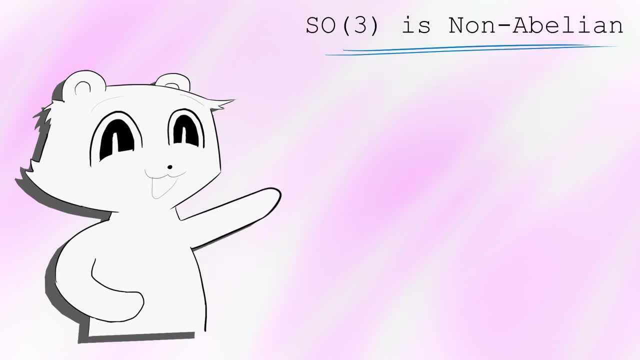 as if I rotated 60 and then 20.. Meanwhile in SO3.. SO3 in three dimensions. The fact that I have different axes means that this doesn't always apply. If I rotate first around the x-axis and then the y-axis, my vector looks different than 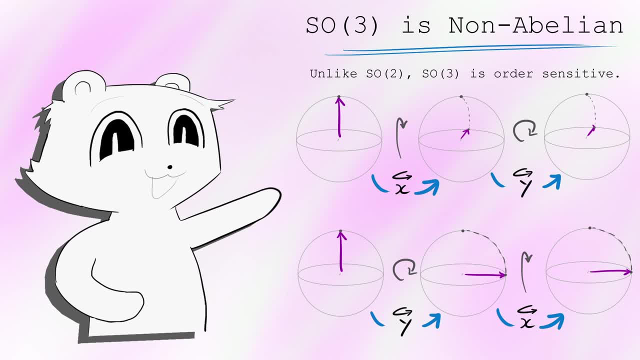 if I were to rotate around the y-axis and then the x-axis. Having to keep track of the order of operations is an important part of non-abelian groups, of which SO3 is one. The U1 symmetry group. The U1 symmetry group. 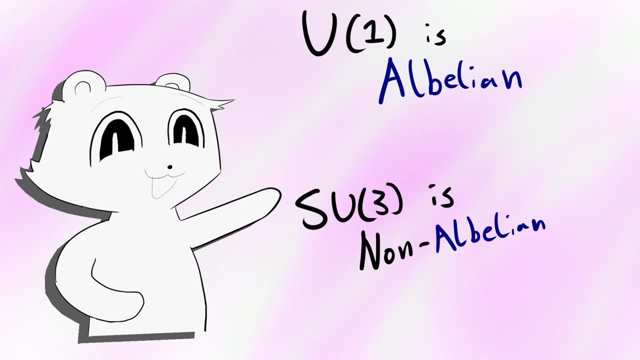 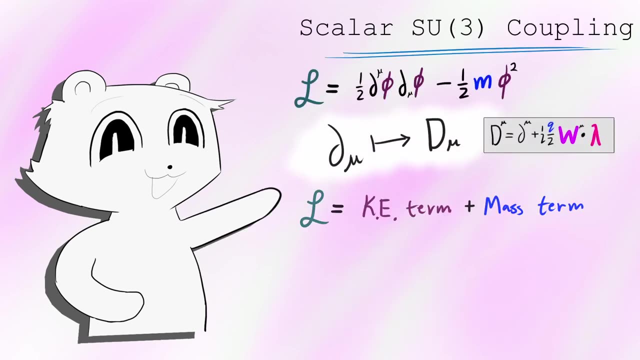 The U1 symmetry group Is abelian, The SU3 group Is not. Because of this terms that would usually cancel each other out- cannot, because mathematically non-abelian group terms cannot be swapped around. This cannot equal this and therefore we end up with these higher-order self-interaction. 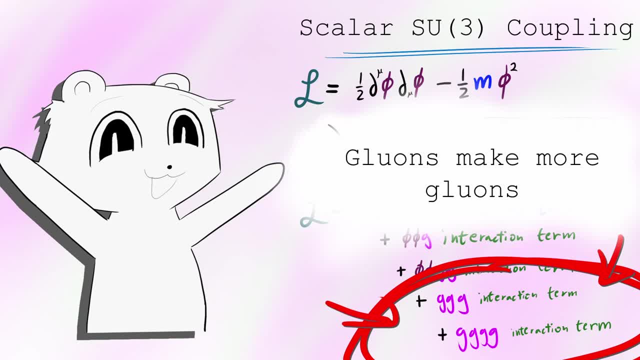 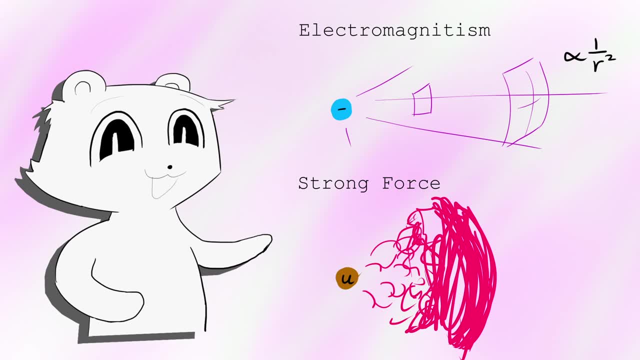 terms in our Lagrangian, and it is these terms that make the strong force so weird: ELECTRO-MAGNETISM. ELECTRO-MAGNETISM: as two charges get further apart from each other, the force weakens by the inverse square law. 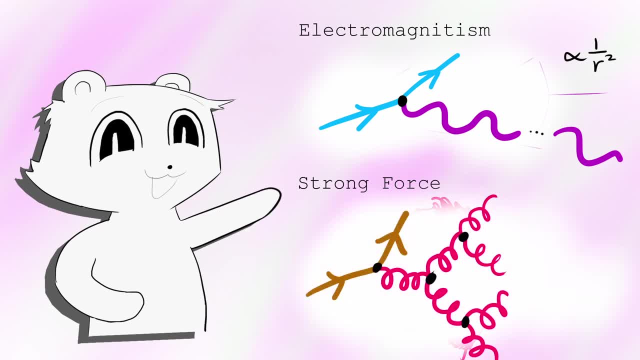 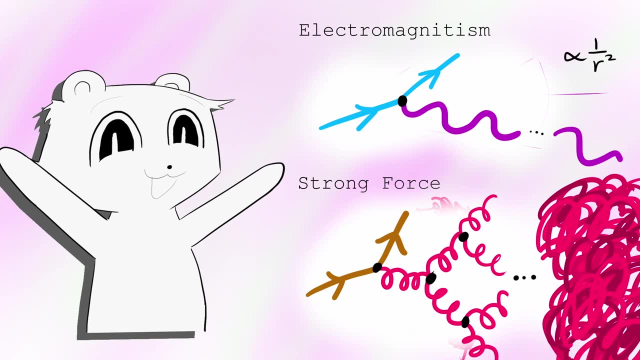 Meanwhile two particles that have an attraction via the strong force. the further they are apart, the more space between the two particles that individual gluons can produce more gluons. Counterintuitively, the force gets stronger and stronger and stronger as you try and separate those two charges. 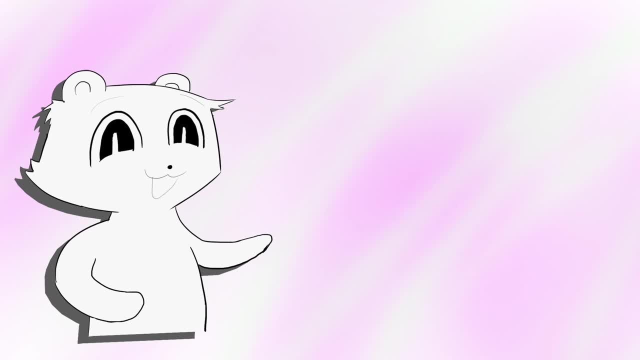 There's a surprising amount that I had to leave out of this video because I tried to talk about the standard model without the mathematics. For instance, how is energy conservation handled at all in these equations? Turns out, because all these equations use spacetime tensors. 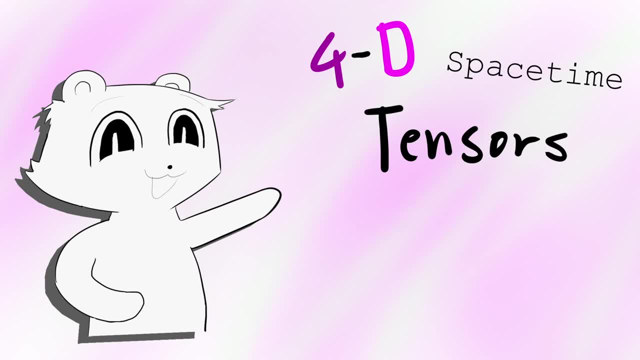 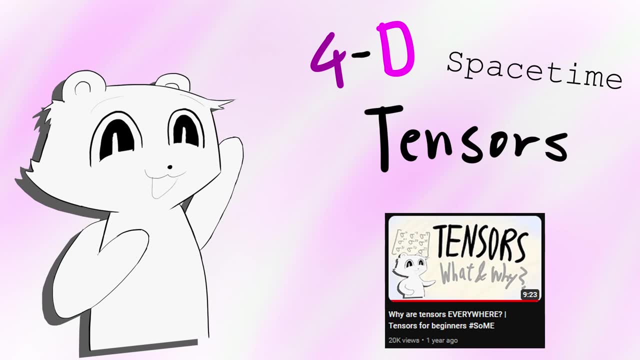 they automatically include special relativity, which deals with energy conservation. You can watch my tensor video to see a bit more on how this is done, but energy conservation being handled automatically is a great feature. I also skipped over perturbation theory, which is the theory that Feynman used. 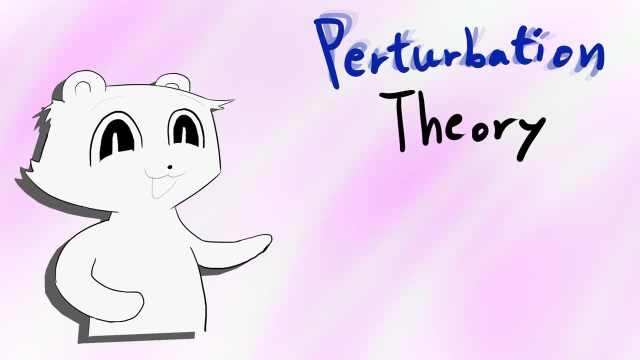 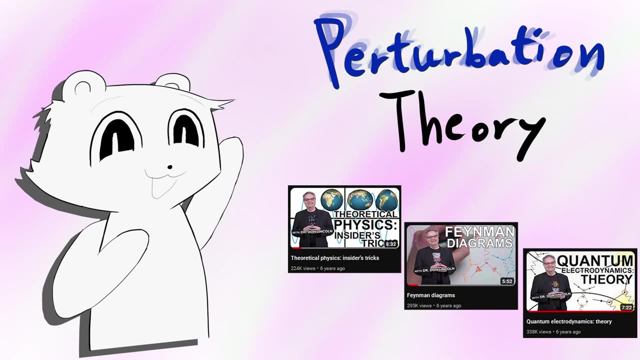 to get his Feynman diagrams in the first place. If you want to actually make discoveries yourself, you have to get terms with perturbation theory and Fermilab's. Dr Don Lincoln has some good videos introducing the concept of perturbation theory. 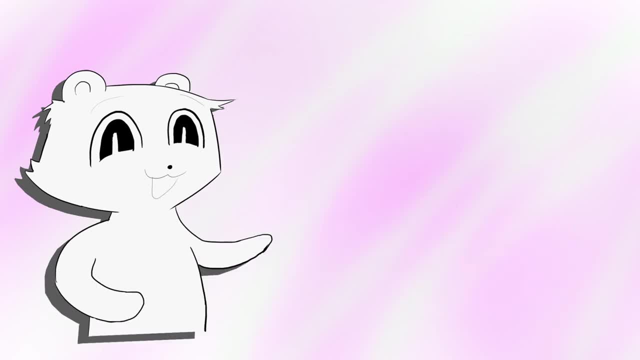 Also, there's no way to avoid the raw mathematics of working in the Lagrangian. I summarized quite a bit in this video and I hope you enjoyed it. There's quite a few things, which is good enough: intuition for the electromagnetic and strong. 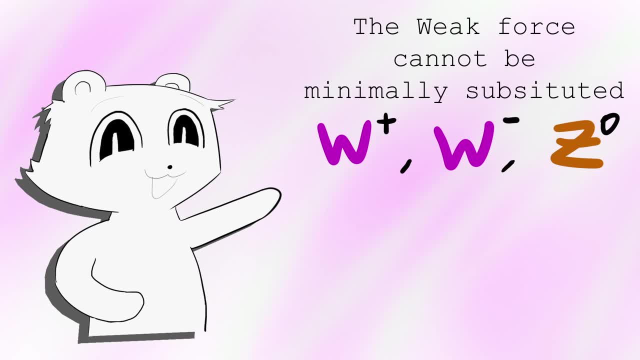 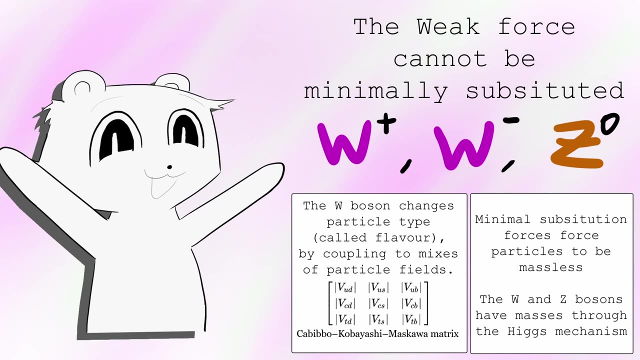 force, but for the weak force it is vital in understanding its two massive exceptions. It couples to the mixes of fields determined by the CKM matrix and is the only boson field to have mass that is attained through the Higgs mechanism. 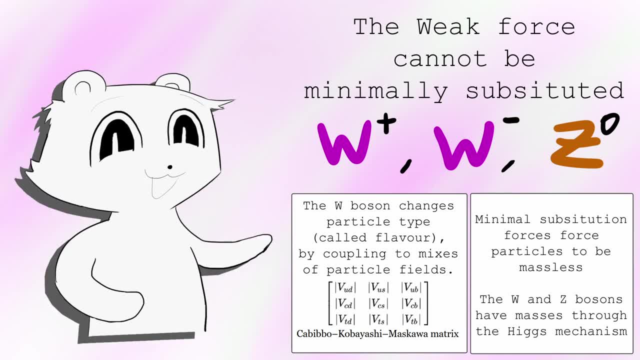 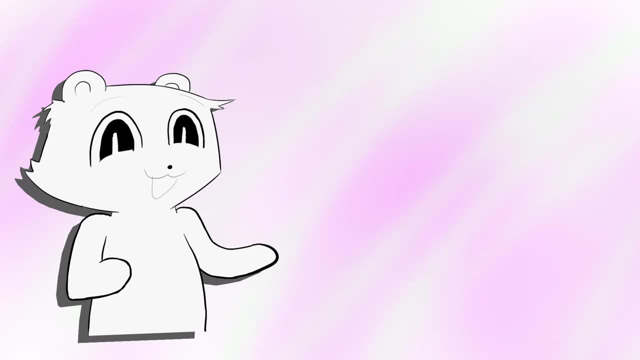 If you want to understand a single word that I just said, you're gonna have to go to university and you, my friend, are gonna have to learn it too. It's very worth it, I'd say. If you found this video enticing, you're exactly the kind of person. 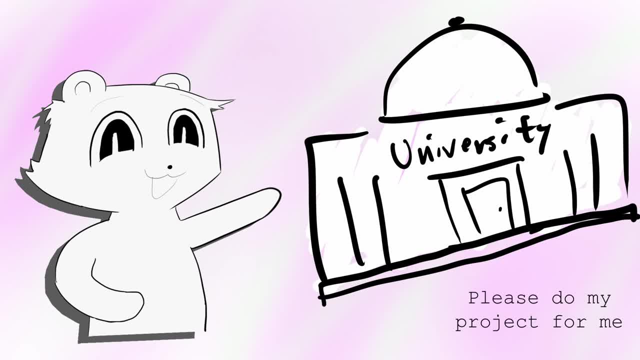 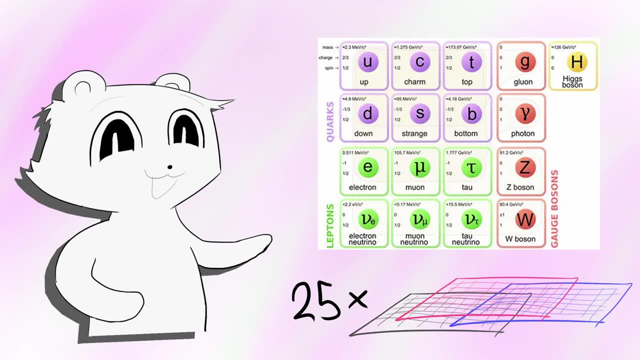 I want at my university learning this kind of stuff. I believe the raw logic of the standard model is gripping and genuinely insightful. There's nothing that arbitrary about the choices behind the standard model. It simply models what we see in the world and uses incredibly fundamental and perspective-shifting logic to peek into the subatomic.